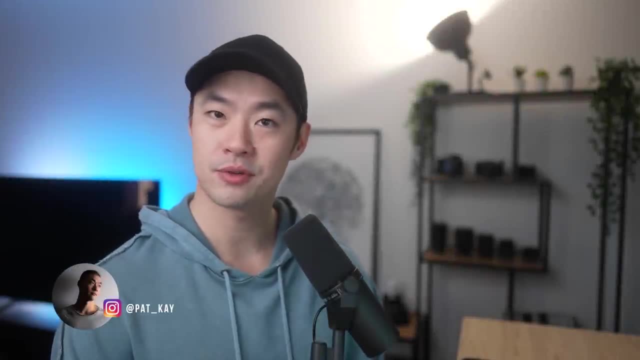 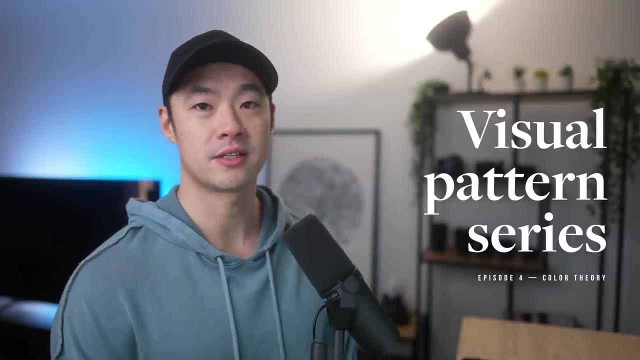 Hello, my lovely photogs, welcome back to another video, Welcome back to the visual pattern series, The series where we break down visual language into visual patterns so that we can understand the heuristics of visual language and how to best apply it to our photography. Now, if you don't know, 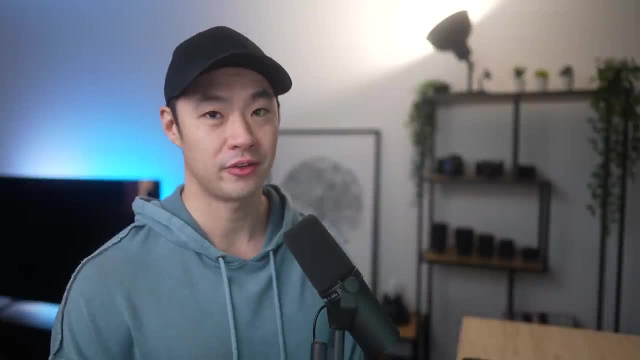 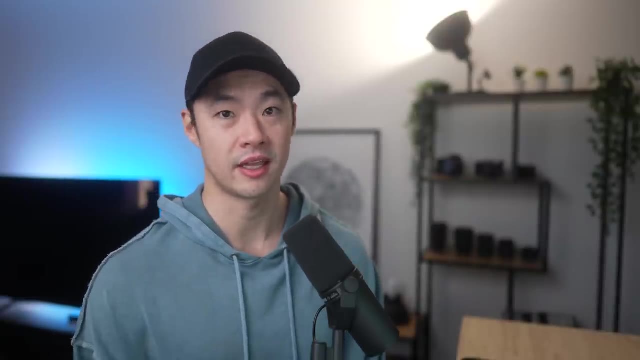 what any of those terms mean. make sure to check out the very first video in the series, where I break down all of those terms and exactly why you would want to use visual patterns over something, say, like photography rules. Now, in this video, we're going to be covering color theory, for 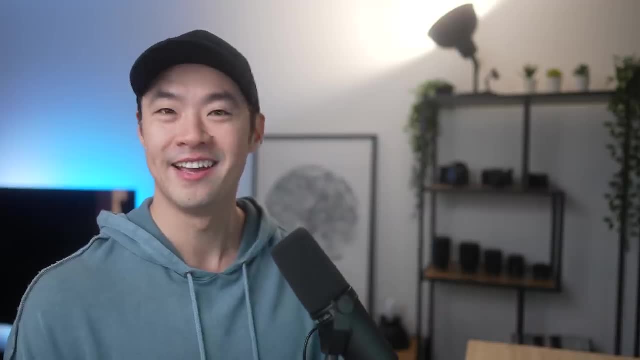 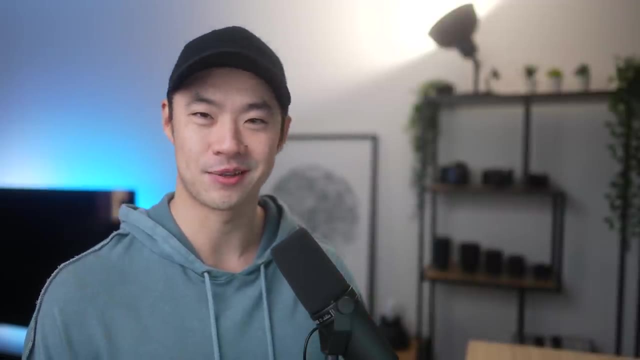 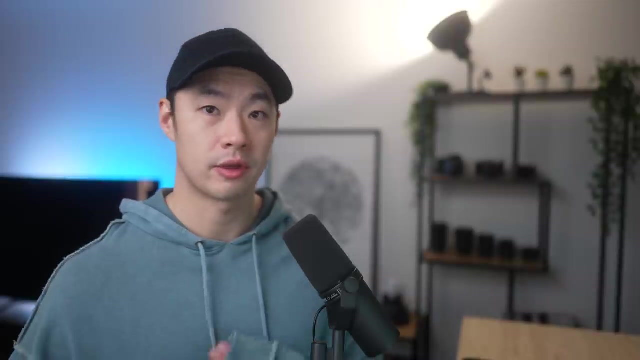 photographers- and this is a an impossibly a large video topic to cover in just one singular video, but we're going to try and do our very best Now. color is a fantastic way to elevate your photography if you use it in a methodical and intentional way. It's not only great for 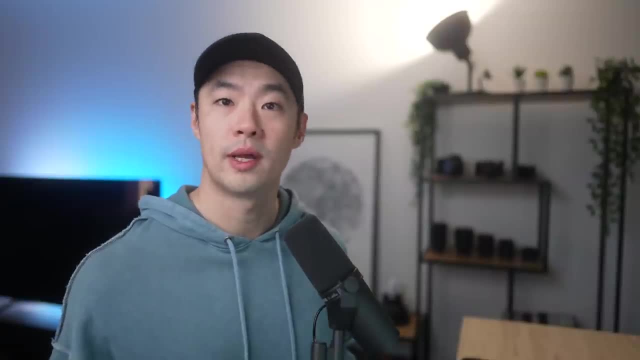 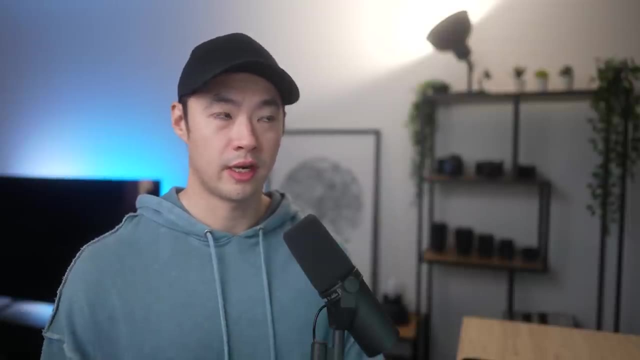 photography, but it's also great across all disciplines of art, So it's a really good skill to understand for your creative process. Now there's a lot to cover and I wanted to start this video with understanding terms, So let's start with hue Now. hue is just. 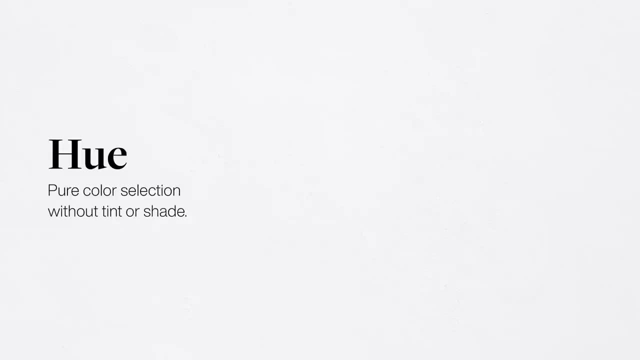 color selection. plain and simple. It is pure color, without the tint or the shade. Some people like to complicate this a little bit, but simply it's just the color that you're selecting and most of the time it's presented on a scale of adjacent colors. 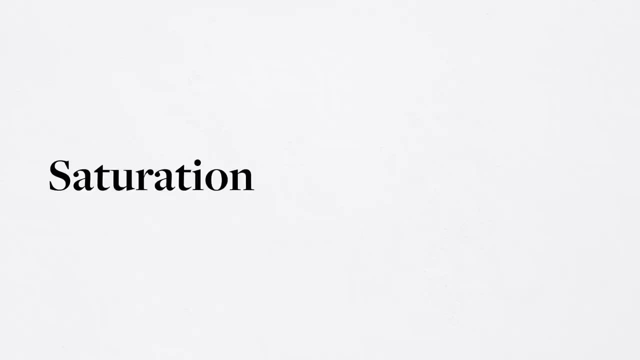 The next term is saturation. Saturation refers to the intensity of color. So once we take a color, do we increase the saturation and make it more intense and more vibrant, or do we make it less saturated and more muted and understated? The next term is luminosity, which refers to how bright 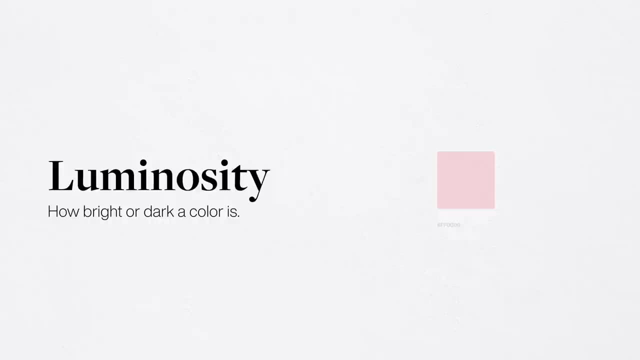 or how dark a particular color is. What we can do is we can add white to a particular color to increase how bright it is, but doing so we can make it more vibrant, and more vibrant will also decrease how saturated it is as well. conversely, we can also take that same base color. 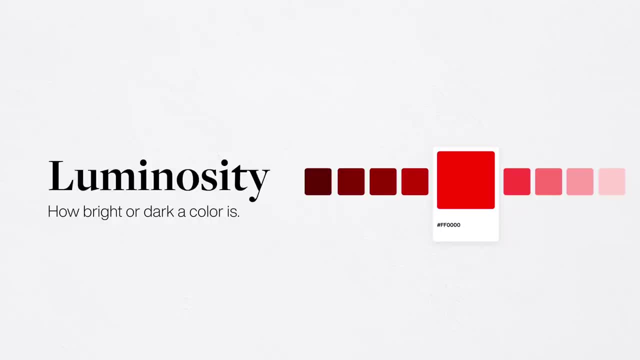 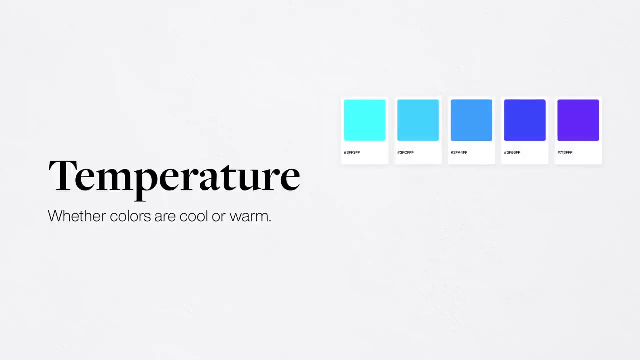 and add black instead to it, making it darker and also increasing the richness of its saturation as well. the next term is temperature. temperature refers to whether colors in general are cool or they are warm. cool colors gravitate towards the color blue, and warm colors gravitate towards the. 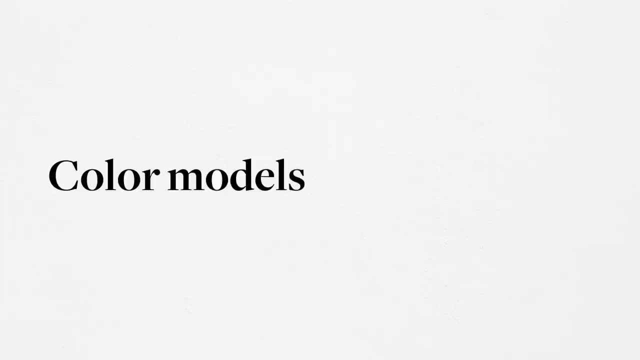 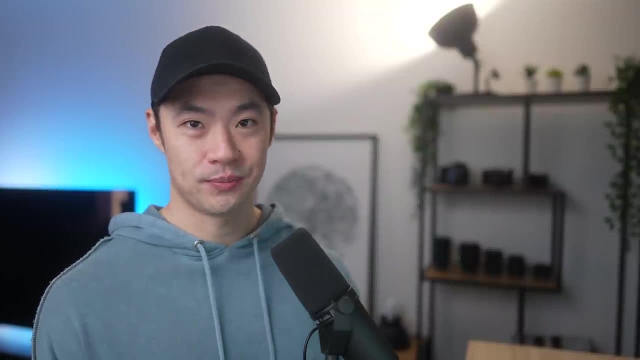 color orange. okay, from here i want to talk a little bit about color models, but this can get really really technical, really really quickly, so i will try and keep it short now, unlike in primary school, when you would mix finger paint together, the colors that you would mix together back then. 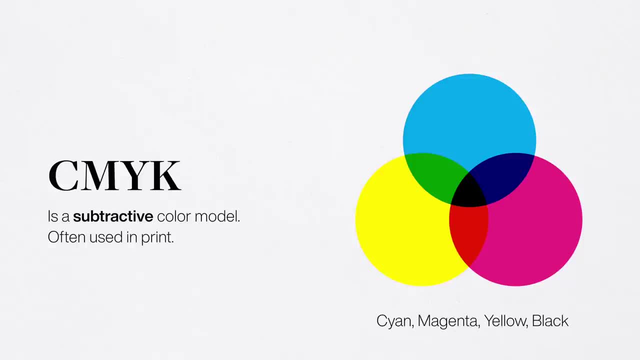 would become darker and they would become more rich, whereas in the digital space, actually the opposite is true. in the digital space, we work with a color space called rgb, and that doesn't actually work, as well as in the digital space, we work with a color space called rgb, and that. 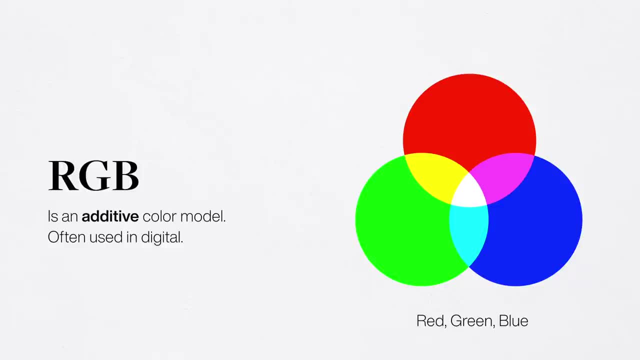 doesn't actually work this way. you might have heard of rgb before, or you might have heard of srgb as the color space before. what this means is that because we work on screens, when we're taking digital photographs and we're looking at monitors and what have you? the screens actually. 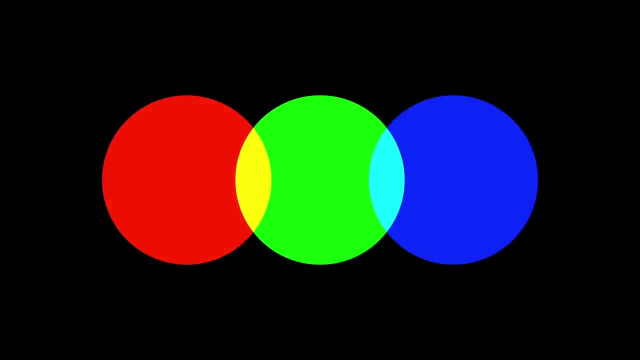 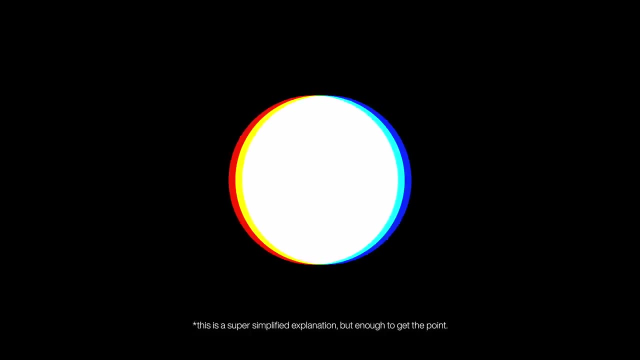 project light at us. each color- red, green and blue- is an individual light and when the lights are combined together they equal more light until you get eventually white. now the whole thing about rgb gets a whole bunch more complicated than the actual color space, so we're going to talk a little bit. 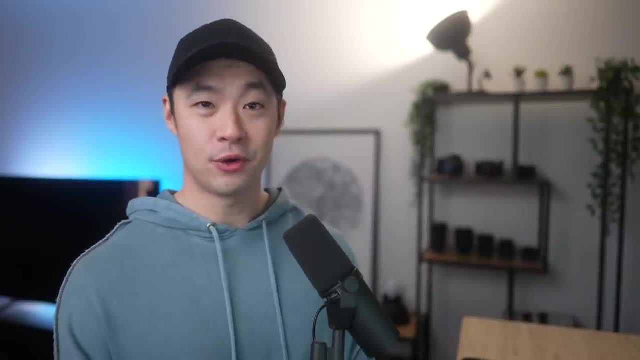 more about that in a bit, but that's another video for another time. all you really need to know is that, as a photographer, you will be using the srgb color space and we'll be working in rgb colors. all right, now we get to the interesting part: color psychology. now these are objective truths. these 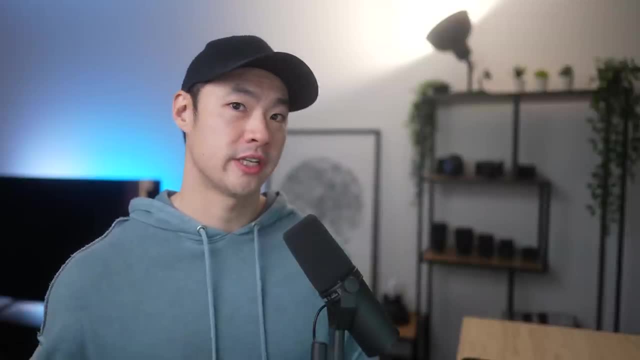 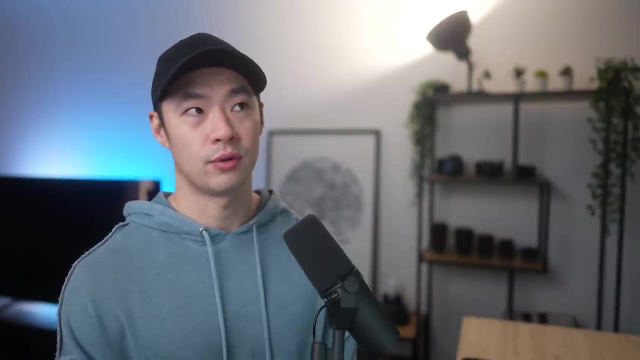 are not subjective truths, although they do have some subjective variants to them. the psychology of color has been greatly studied for a very, very long time now, and i'm going to talk a little bit more about that in a bit. but first let's talk about subjectivity and what it means to be a color. 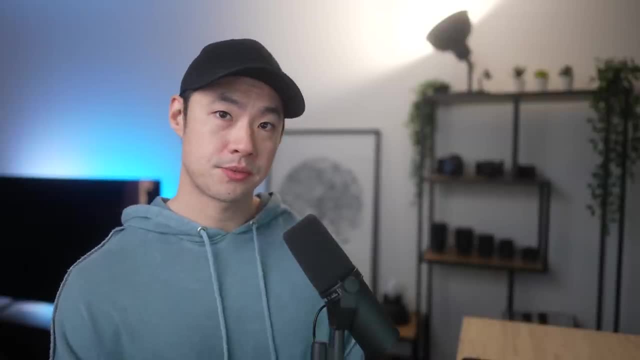 and so a lot of these ideas are well established and have been proven. but, as i mentioned about subjectivity, some of these colors have different meanings for different people, depending on what kind of culture you're from, depending on what kind of background you have, depending on external. 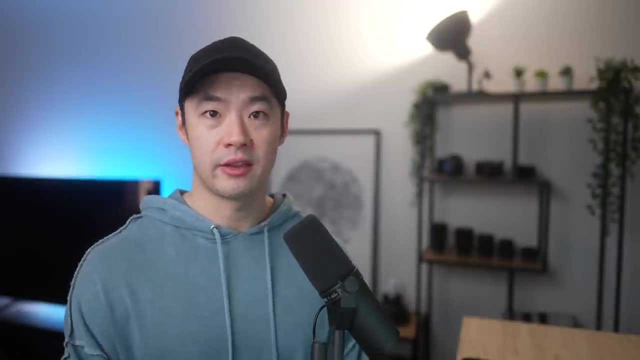 factors like branding and how submersed in that particular brand you are and what that means to you, things like upbringing, things like environment- a whole bunch of external factors can change the overall subjectivity of what these colors mean to you, but in general it's a lot of different things. 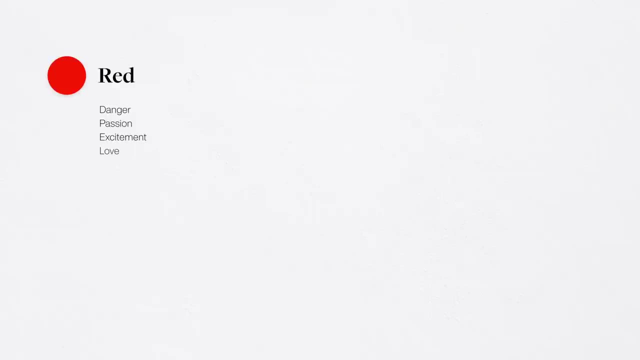 so we'll talk about that in a bit, but first let's talk about what these colors mean. well, these are what the colors mean. red is the color of danger, passion, excitement, love and energy. orange is the color of creativity, of happiness, friendliness and confidence. yellow is the color of warning, optimism. 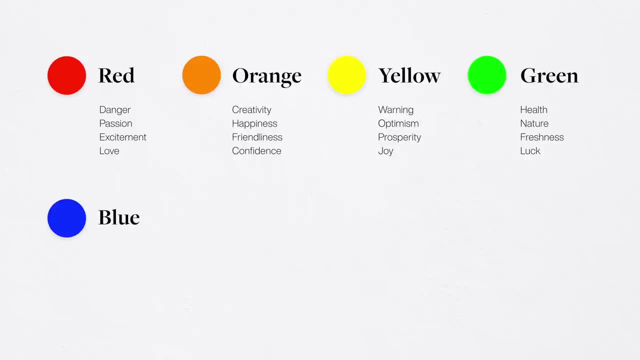 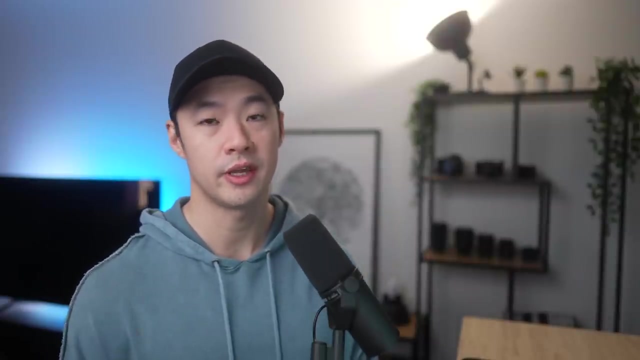 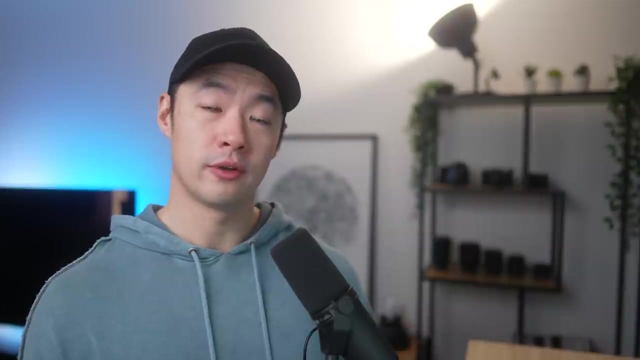 prosperity and joy. green is the color of health, nature, freshness and luck. blue is a color of calm, serenity, trust and reliability. purple is the color of luxury, wealth, virtue and comfort. black isn't a color of. we know all of the meanings of these colors. what we can start to do is actually group them together. 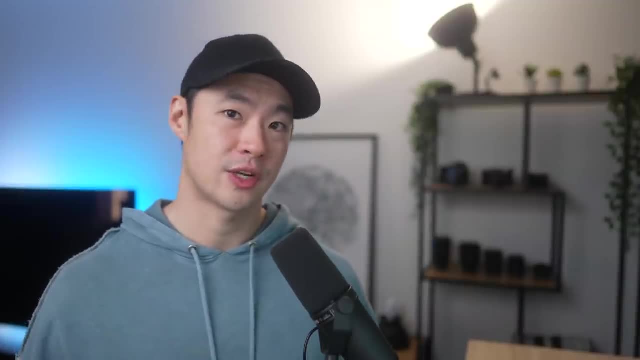 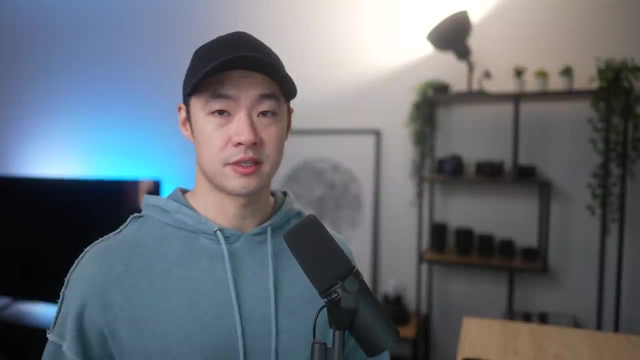 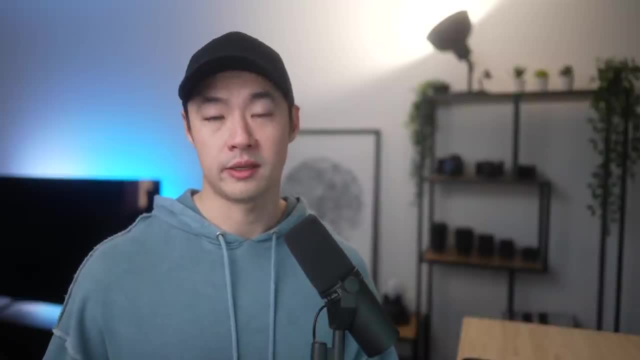 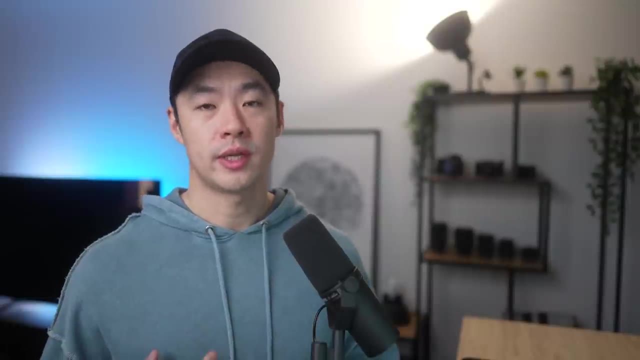 that look visually appealing, and there are some ways that are more appealing than others. Now, what we can do is start to gravitate towards a particular palette that we create, and we can start to accentuate this palette within our photography, Now, a tool that I love using when it comes to color and understanding. 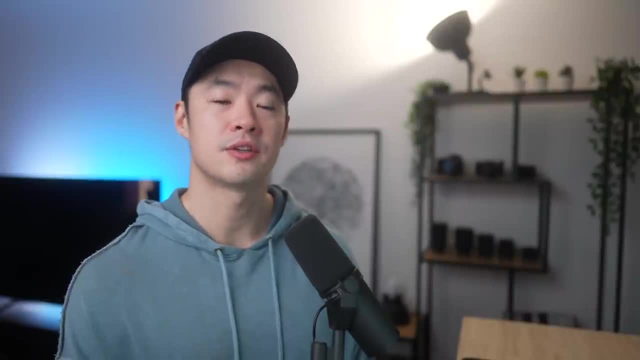 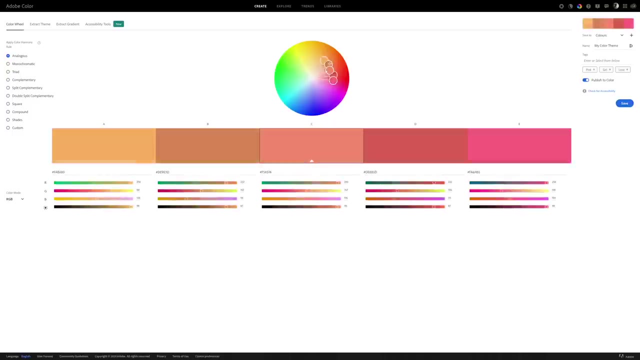 color harmony in general. just playing around with all these different colors is called Adobe Color. I love this tool. I've used it for over 15-ish years in my previous career and it's still something that I use to this day. This is not sponsored, but it's just a product that I love. that's free and you can play around. 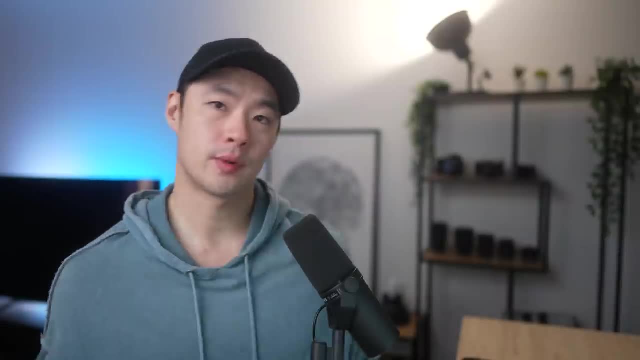 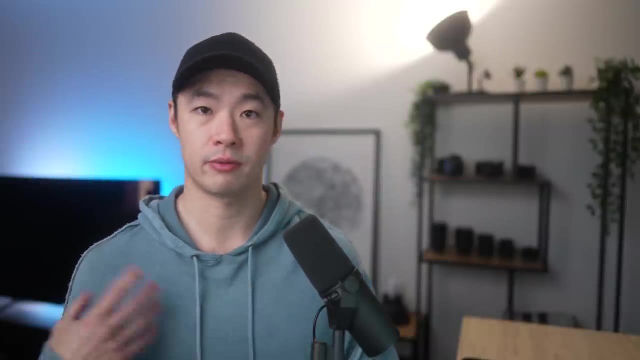 with all the sliders and palettes and all that kind of stuff, and it's great. So what I want to do is introduce you to three of the most common color harmony groups so that you can get a good understanding of those and then from there you can dive into different color harmony groups if you would like. Now the three color harmony groups are called Adobe Color. I love this tool. I've used it for over 15 years and I think it's a great tool to get a good understanding of what color harmony looks like. Now, the color harmony groups that we have commonly in: 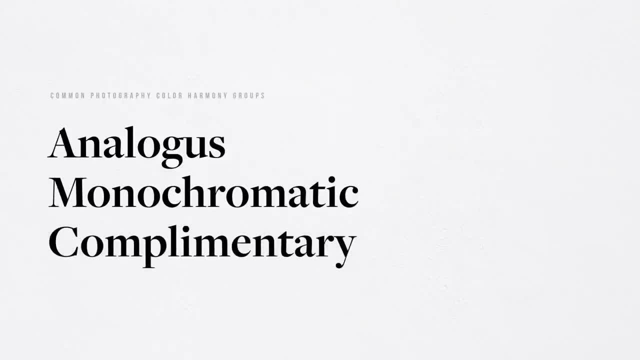 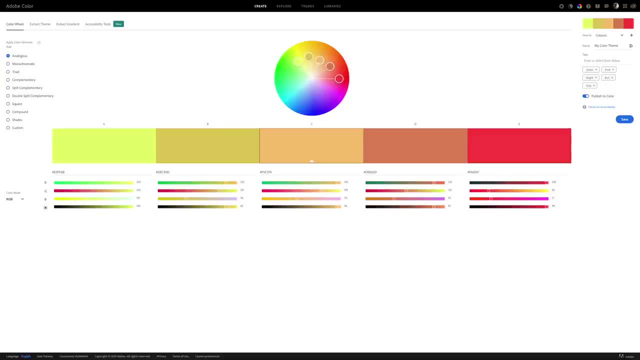 photography are analogous, monochromatic and complementary. The analogous rule is three or more hues that are evenly fanned out from a key middle color on the wheel. You can often find these color schemes in nature, especially in things like sunsets or gradients of the sky or the texture of the ocean, and so so much. 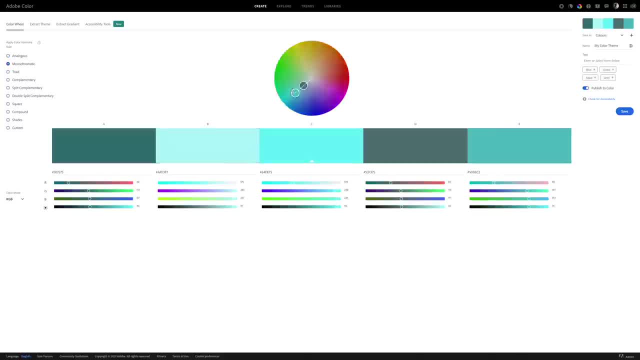 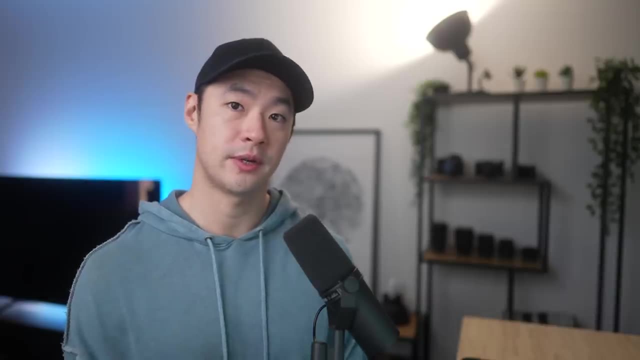 more. The next common color harmony rule is monochromatic, which uses a single key color and accents it with colors of different saturation and different luminosity. This is super, super easy to use in photography, both to find in the world and to edit in post-production. And the last common color harmony group that I want to: 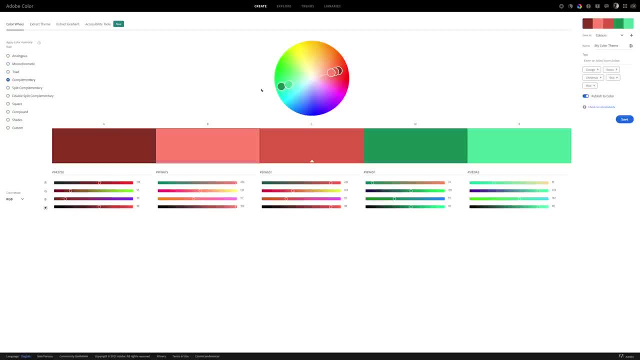 introduce you guys to is complementary. The complementary color harmony rule takes a key color and supplements it with the opposite color on the wheel. This creates a color contrast which is quite appealing and because of the contrast stands out quite a lot. Now you'll see this color harmony group in film, in movies, in photography- pretty. 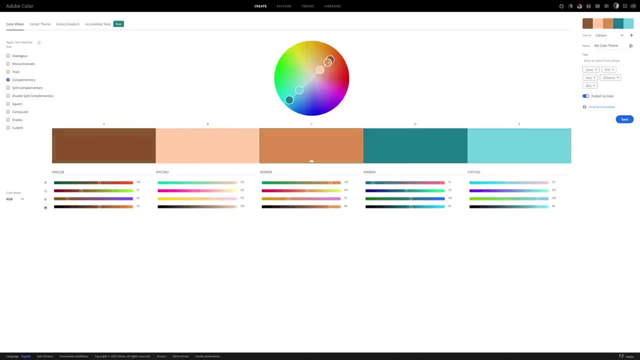 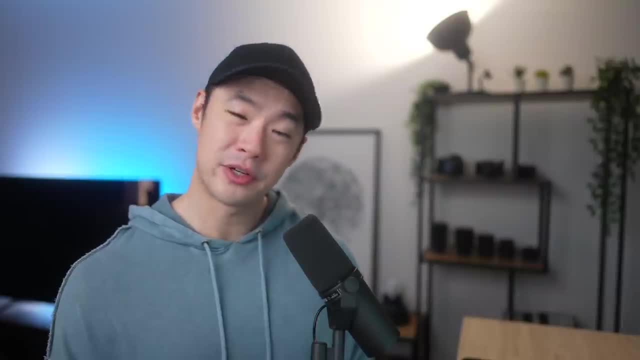 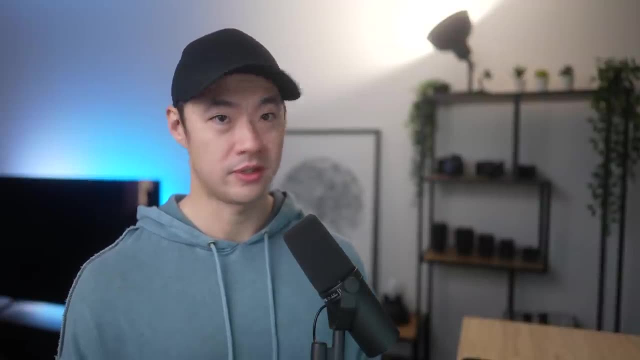 much everywhere nowadays, and the most common color selection from this particular group is teal and orange right now. Now, as I mentioned, there are, of course, a bunch of other different color harmony groups here as well, so feel free to dig into any one of those. there is no right or wrong answer on how. 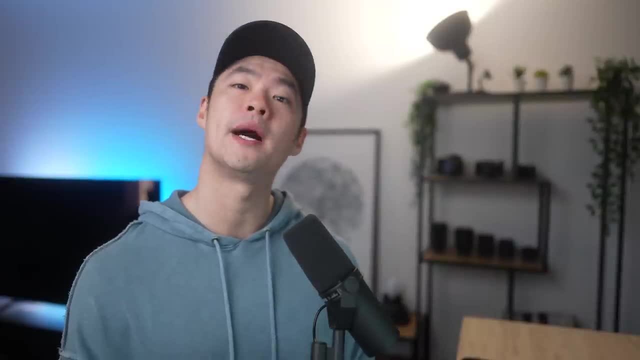 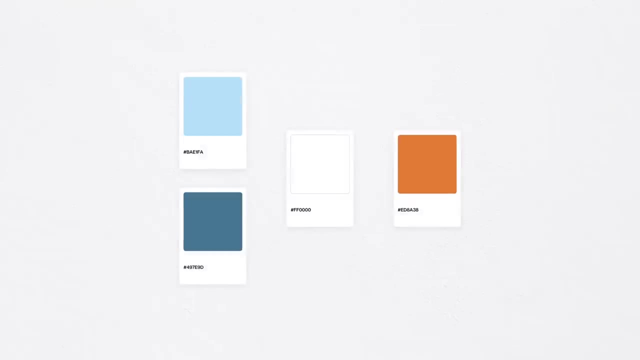 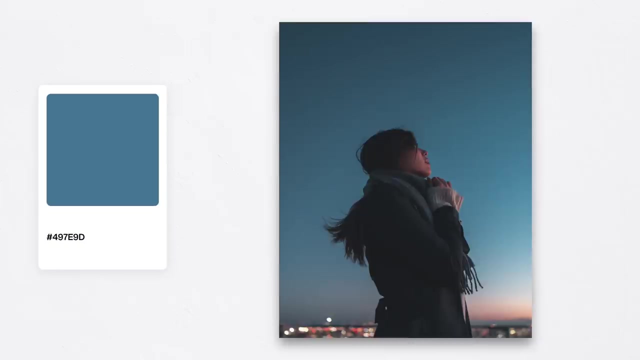 to use different color harmony groups. it's just a suggestion of a palette that you may or may not be able to apply to your photography. Now for me and my photography. I play around with three different colors. I play around with like a kind of between a light baby blue to a cobalt blue and then a lot of white and 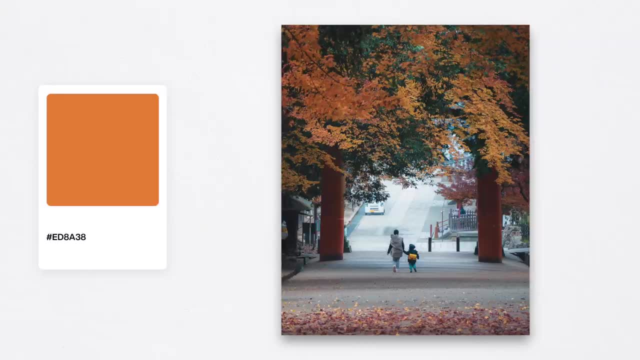 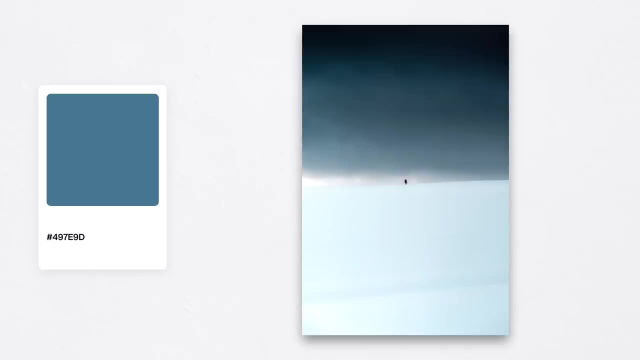 then a lot of orange. So oftentimes I'm actually using analogous colors when it comes to my orange, and for the blues, I'm tending towards a monochromatic palette, with the whites and the blues working together. Alrighty, now that we know all. 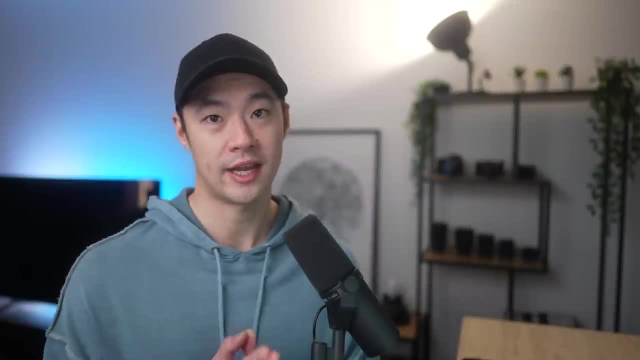 of the colors that we're going to be using in this video. I'm going to go ahead and show you how to use the colors that we're going to be using in this video. Now we can put it all together in something that's actually practical and 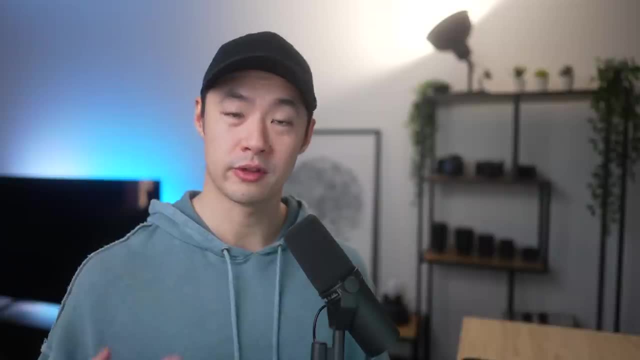 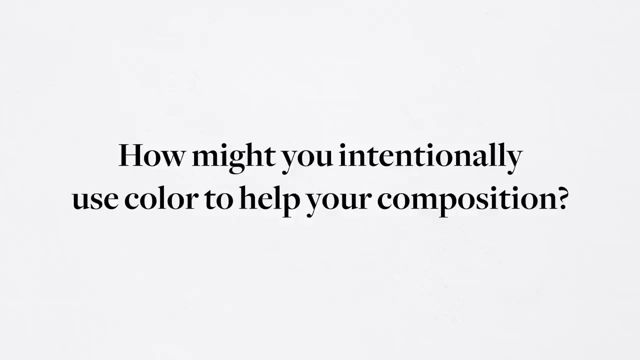 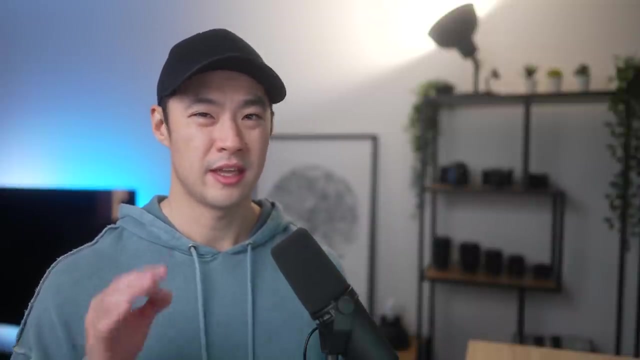 we can actually put into practice Now. when you're out shooting, go and ask yourself when you're shooting, why are you shooting the things that you're shooting, and how can you use color specifically to accent or to bolster or to even help the story that you're trying to tell? Try and push yourself to. 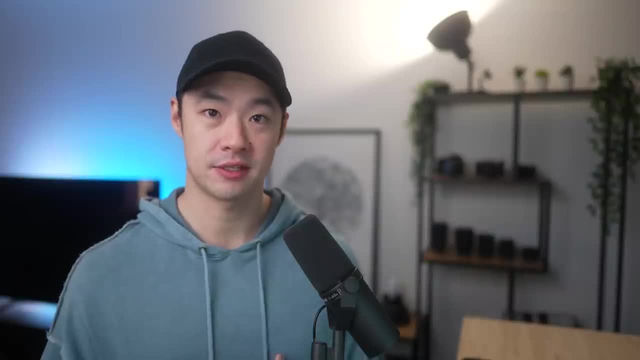 deliberately incorporate color into your work and specific colors, and do it with intention. Now, if you're looking for a habit-based practice, to go out and do yourself- and at the risk of sounding like a broken record, because I feel like I give this advice every single time- but 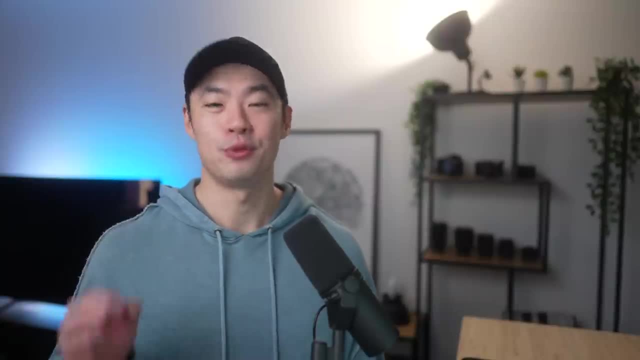 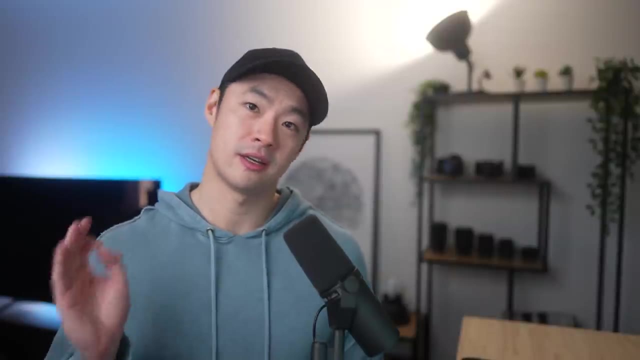 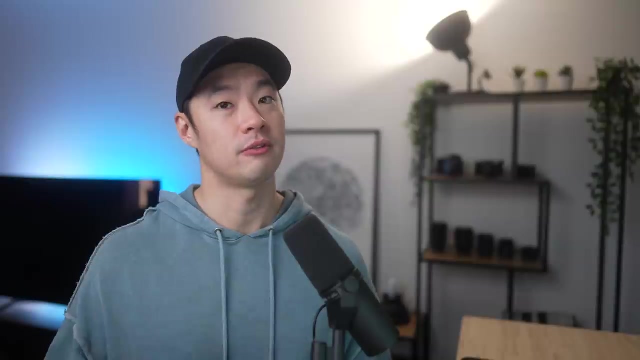 in different ways. spend the entire week with one singular color and shoot that color every single day of the week. Shoot ten of that same color, different compositions every single day, so that you end up at the end of the week with 70 different images of the same color. Now this might sound really simple and 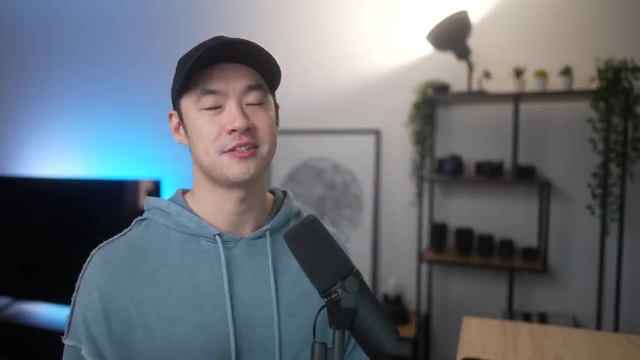 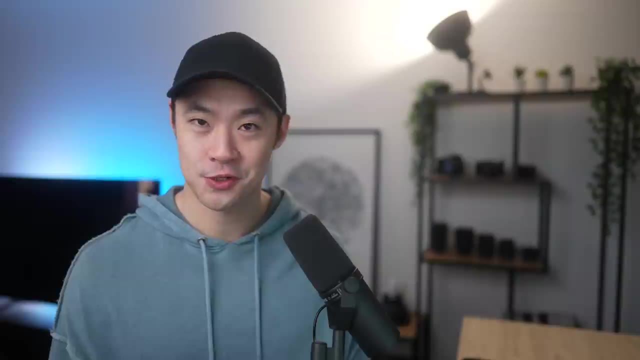 mundane and kind of boring, but I assure you it is extremely difficult. It is very hard and it is going to push you and stretch you creatively in order for you to find these compositions and be able to identify these things in the real world. Now, this practice works really well, and I'll tell you why. When 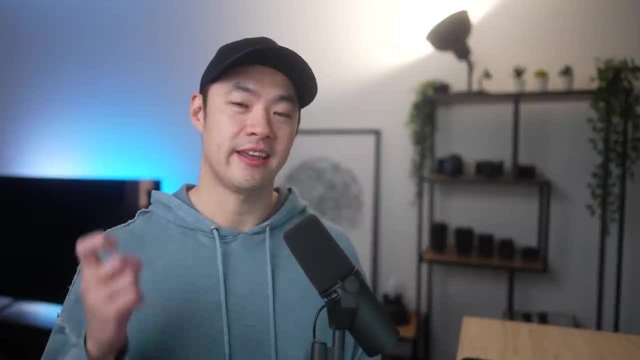 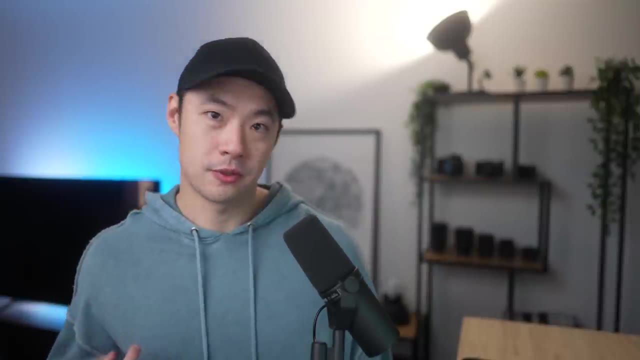 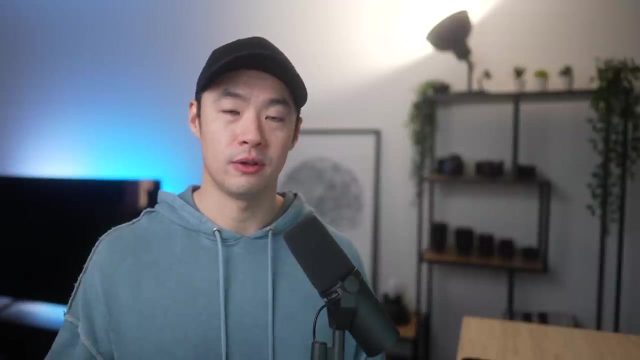 you physically get out there and physically take that image that burns that particular item of that composition into your subconscious. so at the end of the week you'll end up with 70 different compositions that you can quickly recall for that particular color when you need it. you might not need it now. you. 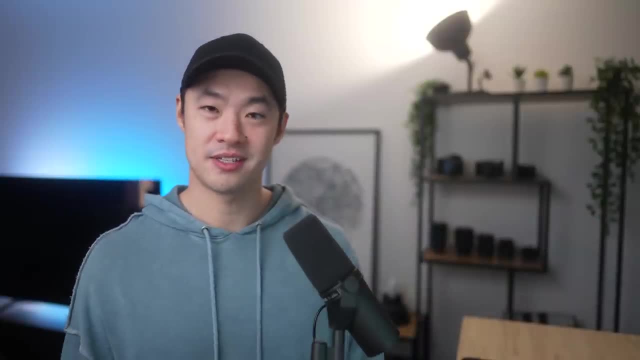 might not need it next year, you might not even need it a couple of years down the road, but knowing these compositions exist, based on this color, is something that's super, super powerful for your recall, for you to be able to use to give meaning and help tell the story that you're trying. 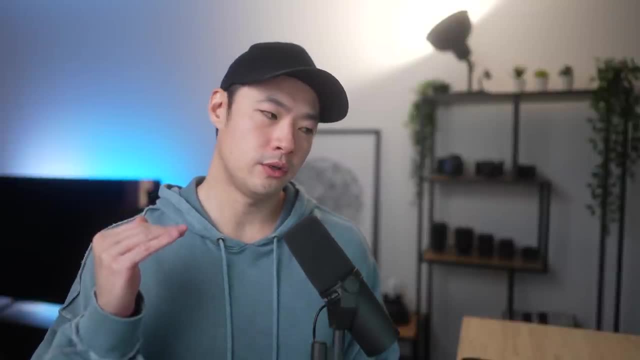 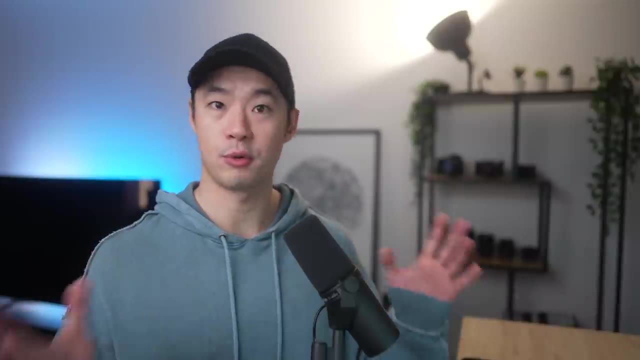 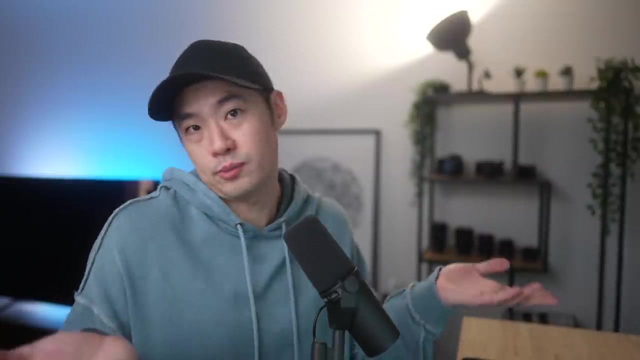 to tell in your photography. now consider this example: you're doing street photography and you decided to pick the color red this week and you find this amazing red brick wall. now people are walking past this wall and you're taking a photo of someone plus this red wall. it would be pretty.